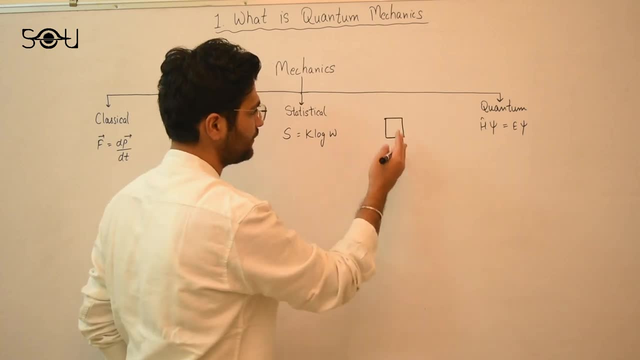 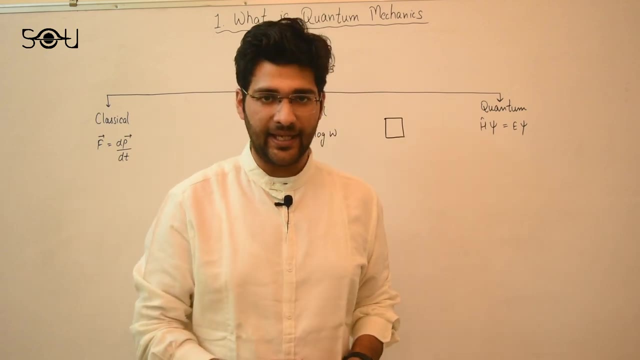 So suppose you have to study a motion, the motion of a box. right, I have drawn this box on the board. Suppose you have to study its motion. Classical mechanics says that if you want to study the motion of this box, all you have to do is to study just one point of this box. 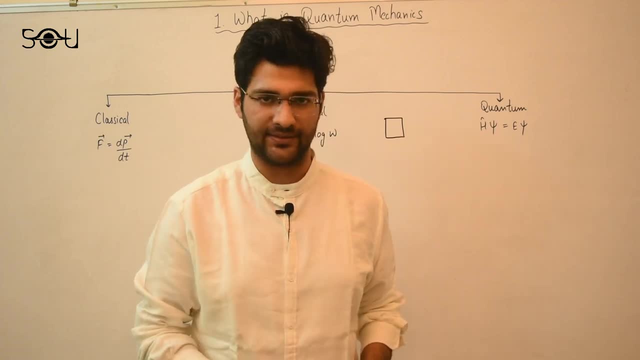 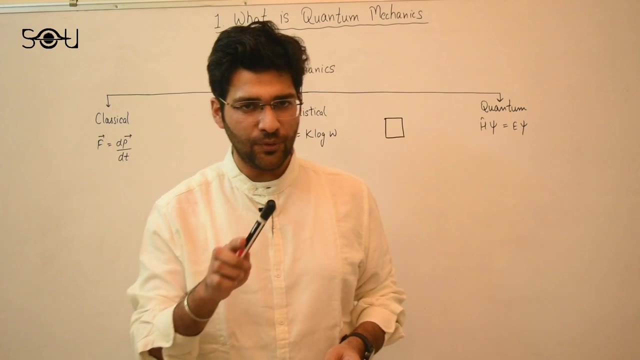 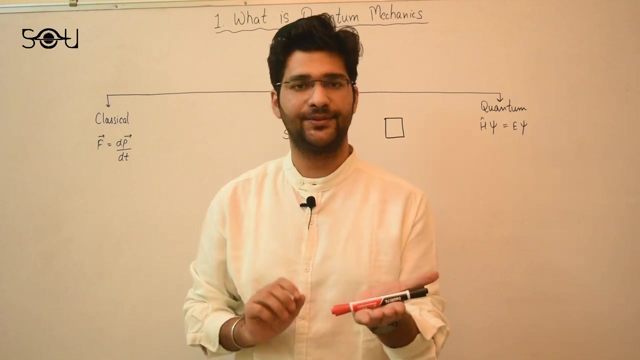 And that one special point is the centre of mass, where all the mass of the box or the body is considered to be present. Let me show you how. Suppose I have this pen in my hand right Now. the centre of mass of this pen is somewhere in the middle of the pen, between the two ends right. 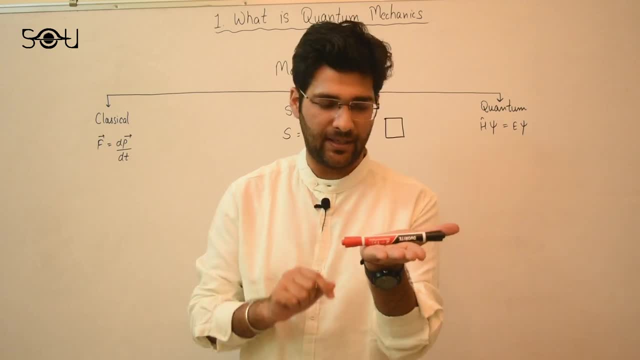 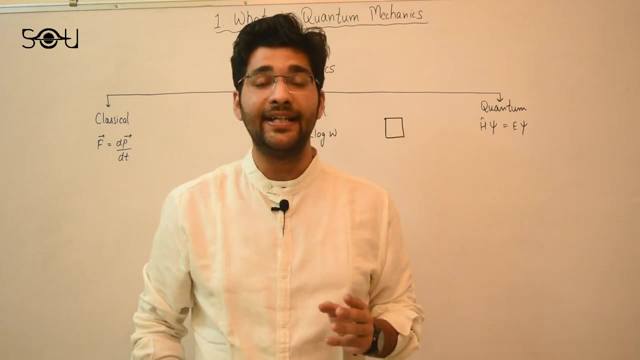 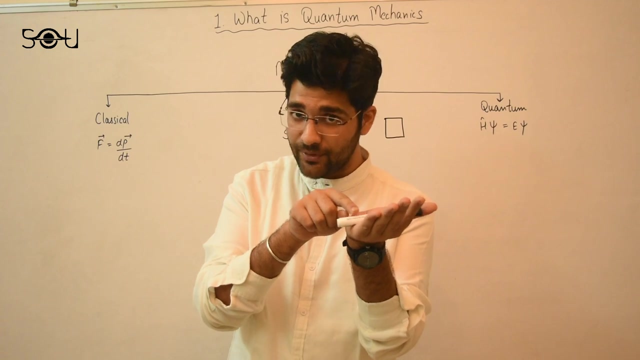 Now watch what happens when I slide this pen across my palm. The pen falls down right. But when does that exactly happen? That happens when the centre of mass of that pen is no longer on my hand right. When the centre of mass is on my hand, the pen is still on my hand. 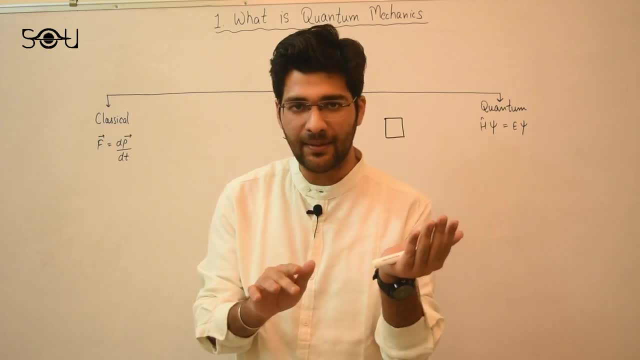 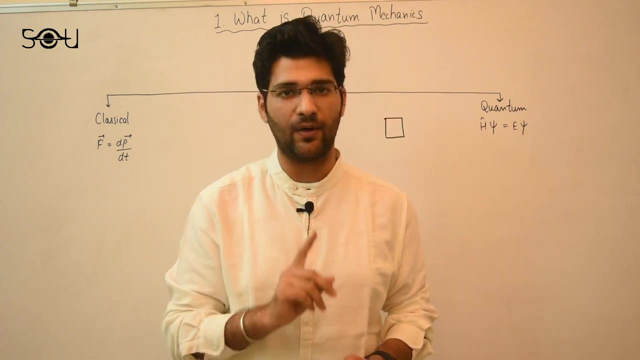 As soon as the centre of mass of this pen slides across my palm, the pen, the entire pen falls down. So you have to study the motion, the equations of motion of just the one point, the centre of mass, and you can study the whole object. 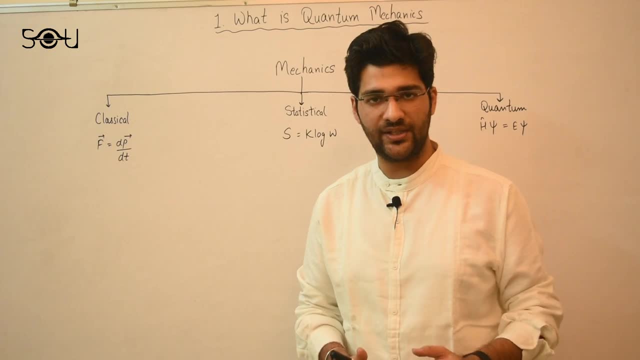 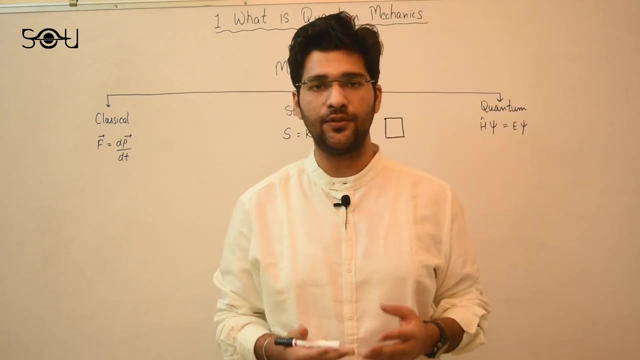 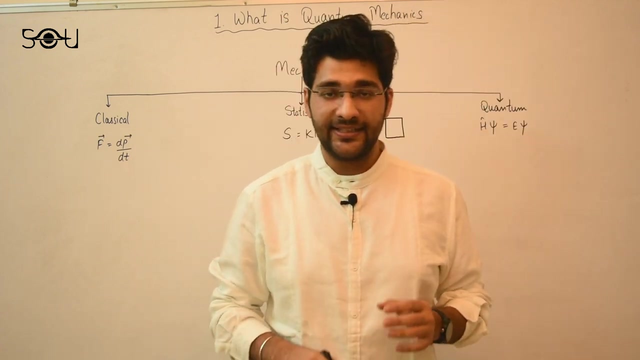 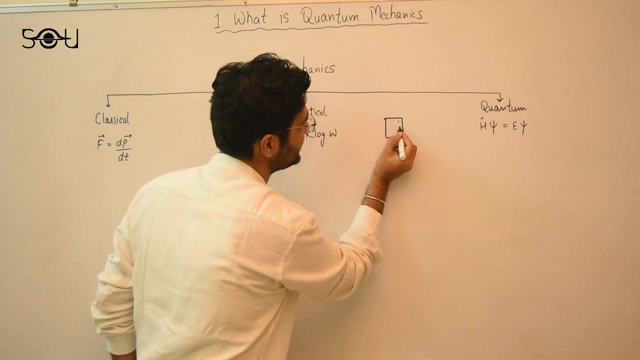 The flagship equation or the most important equation in classical physics is Newton's second law of motion, right, Or you can also use the Hamilton's laws of motion. Now. second is statistical mechanics. Statistical mechanics dives deeper. It says that if you want to study this box, you have to study the motion of each and every particle that comprises this box. 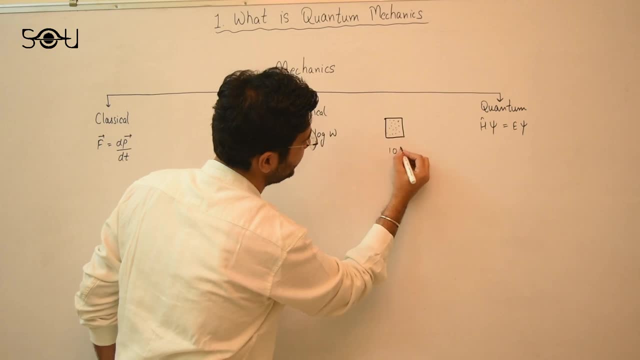 So let's suppose there are 10 raised to power 20 particles present inside this box. So let's suppose there are 10 raised to power 20 particles present inside this box. So let's suppose there are 10 raised to power 20 particles present inside this box. 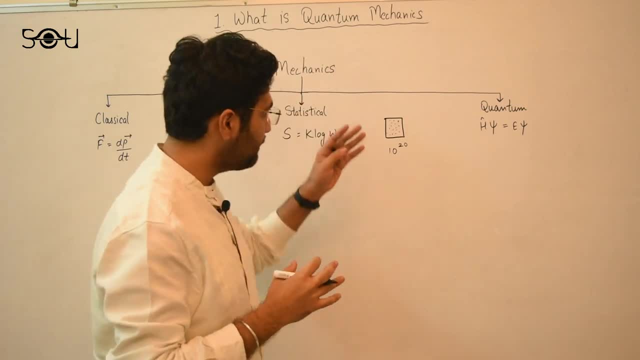 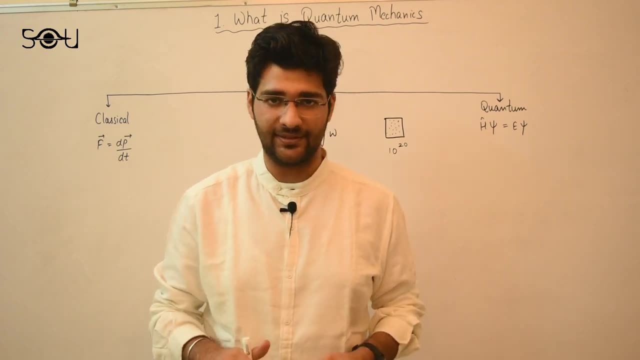 So you will have to gain the knowledge of all the parameters of all these particles. So you must know their momentum, their velocities, their energies of all the particles right. Doing that is practically impossible. Why? Because there are so many degrees of freedom involved. 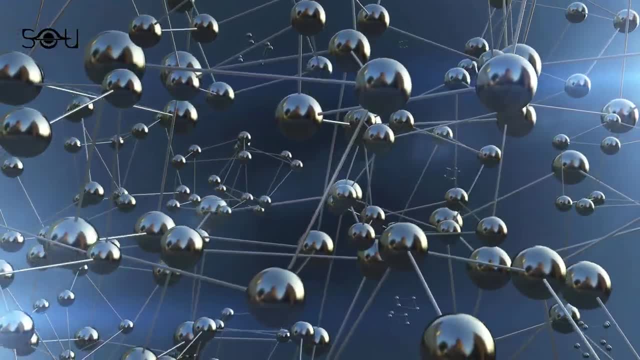 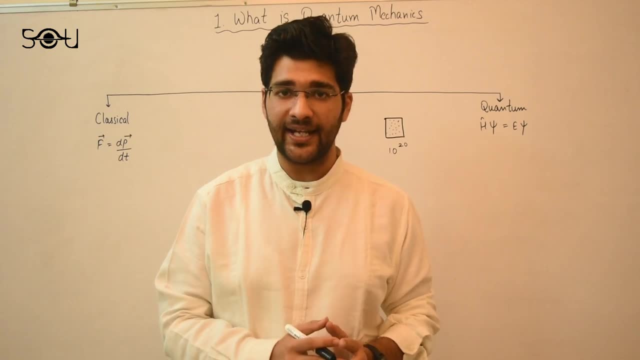 So suppose you have to study a collection of atoms or molecules which is called an ensemble. This is where the ideas of statistical mechanics come into picture. This is where the ideas of statistical mechanics come into picture. In statistical mechanics we generally deal with averages and approximations, because there are so many particles involved. 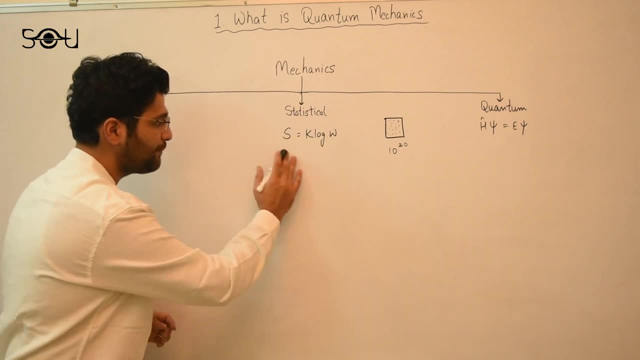 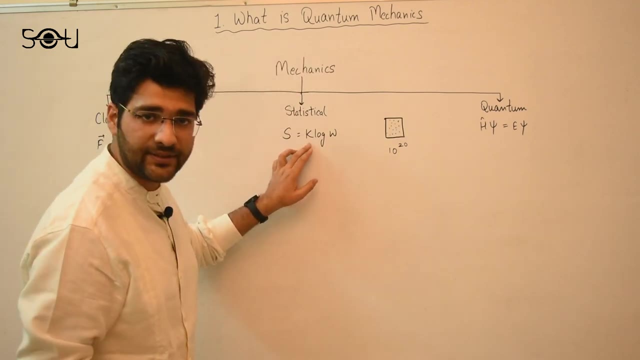 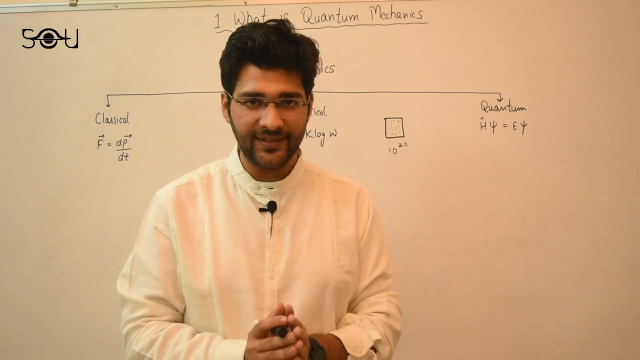 The flagship equation of statistical mechanics is Boltzmann's entropy formula, s equal to k log w, where s is the entropy, k is the Boltzmann's constant and w is the number of microstates present in a system. Now, quantum mechanics, the third type of mechanics, is completely different from classical and statistical mechanics. 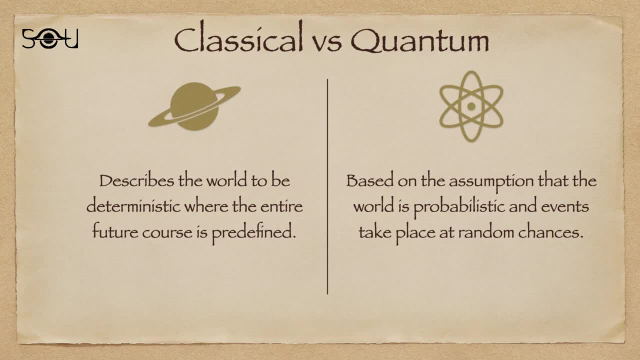 Now quantum mechanics. the third type of mechanics is completely different from classical and statistical mechanics. Now, quantum mechanics, the third type of mechanics, is completely different from classical and statistical mechanics. So if classical physics describes the world to be deterministic, where the entire future course is pre-decided, 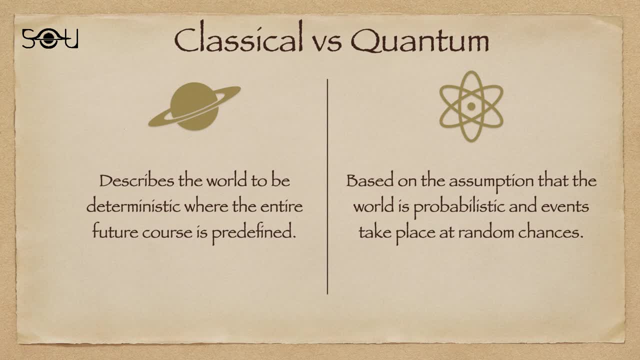 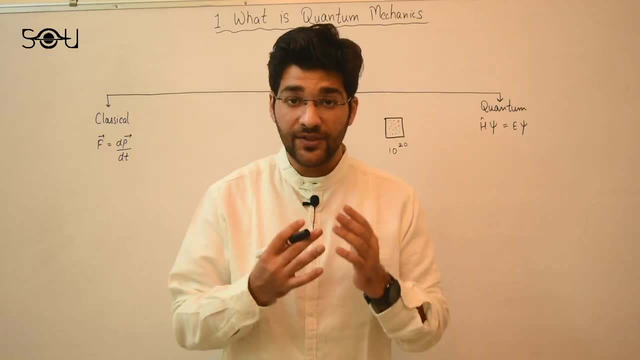 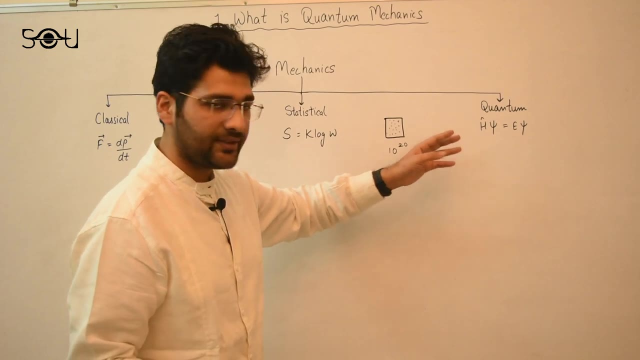 quantum mechanics is based on the assumption that the world is probabilistic and events take place at random chances. The most important quantity which we deal with in quantum mechanics is the state of a system, or the wave function, And the most important equation, the flagship equation of quantum mechanics, is the Schrodinger's wave equation. 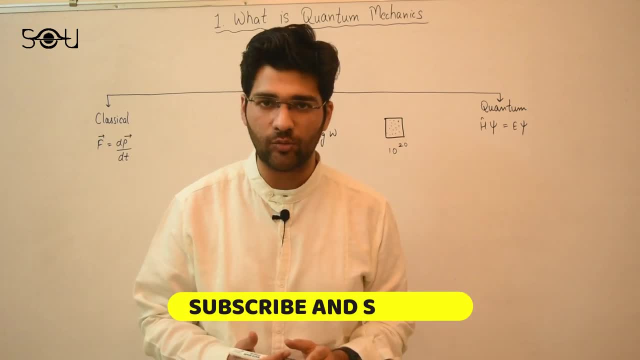 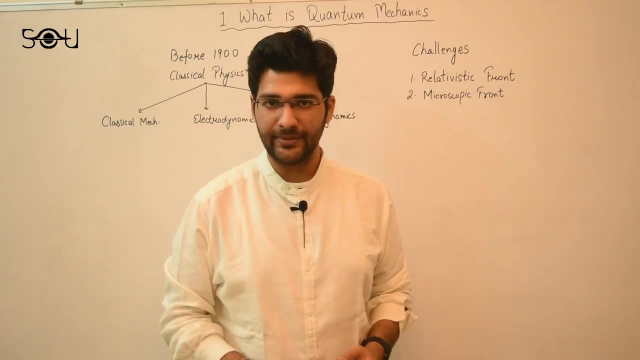 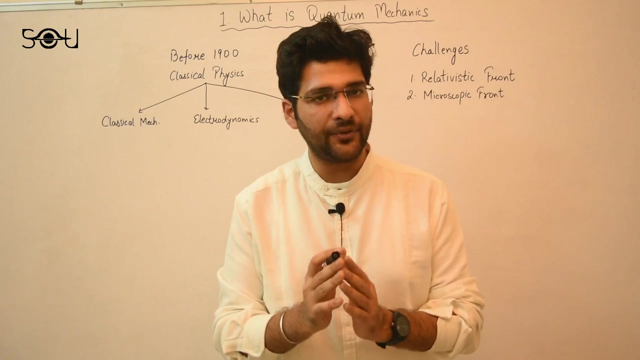 or you can also use the Dirac equation, which is relativistic, unlike the Schrodinger's wave equation. Now let me give you a very brief overview of how quantum mechanics was born. Before the year 1900, that is, at the end of the 19th century, physics comprised three major fields. 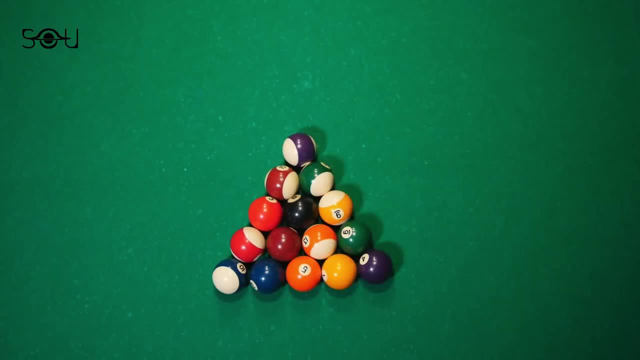 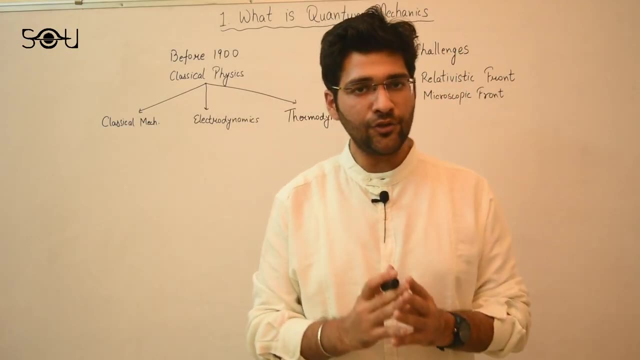 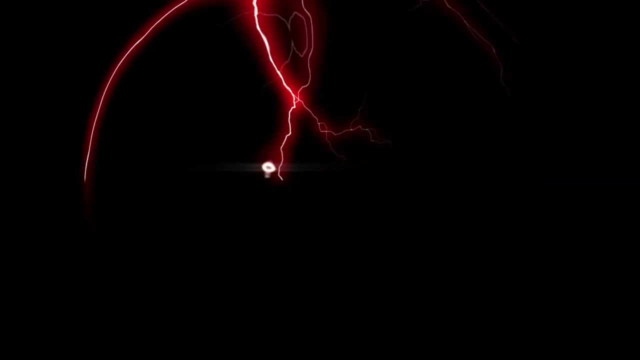 They were classical mechanics to explain the motion of the objects around us. It was based on Newton's laws of motion. Second was electrodynamics. Electrodynamics described radiation. We had four Maxwell's equations that described the relationship between electricity and magnetism. 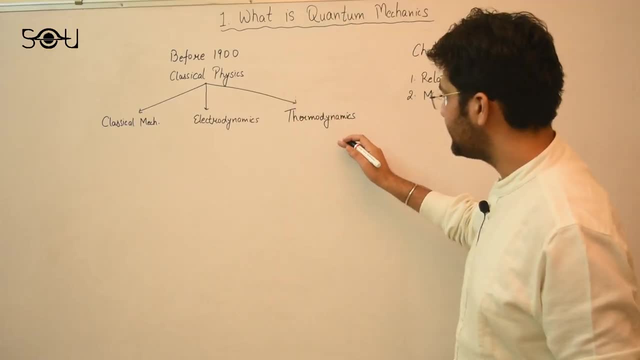 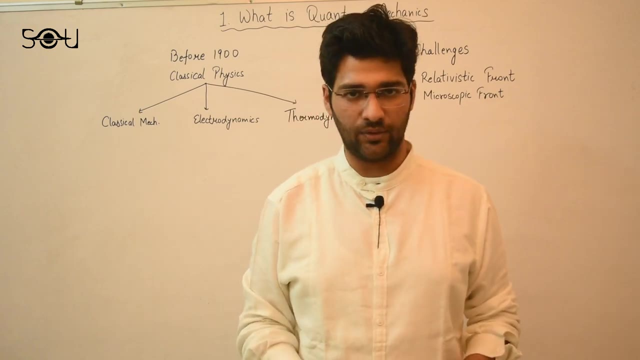 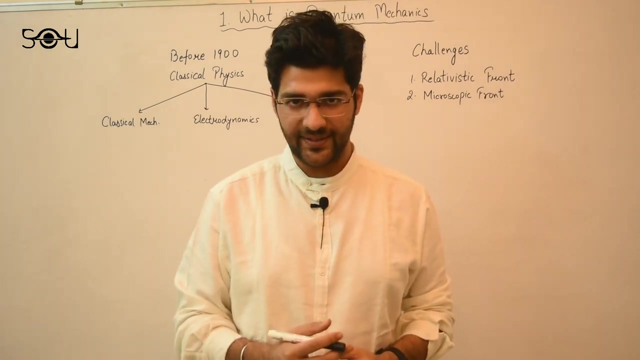 And the third was thermodynamics. that described the flow of heat. So using these three fields of physics, we could explain almost everything around us. So mankind thought they had pretty much figured out everything. However, in the first quarter of the 20th century, that is, from 1900 to 1925,. 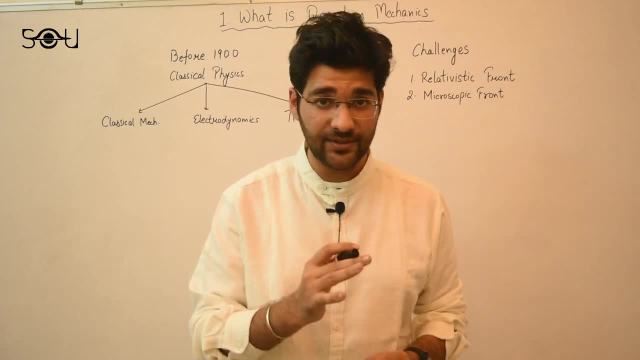 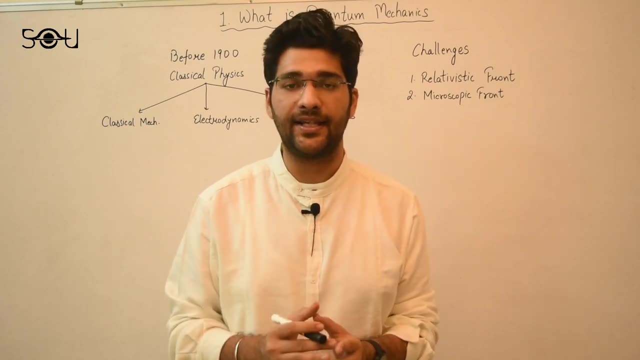 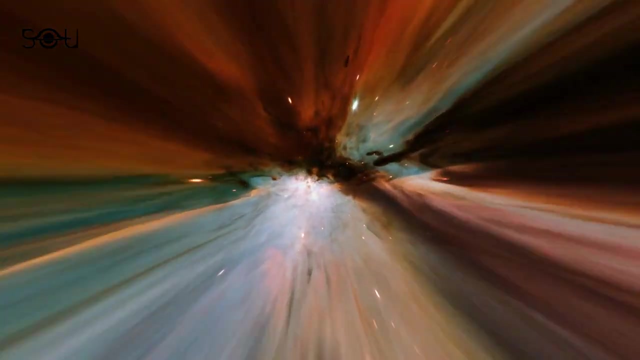 classical physics was born, And classical physics experienced major challenges. The first was on the relativistic front, When, in 1905, Albert Einstein figured out that Newton's laws of motion are no longer valid at relativistic speeds, That is, speeds close to the speed of light. 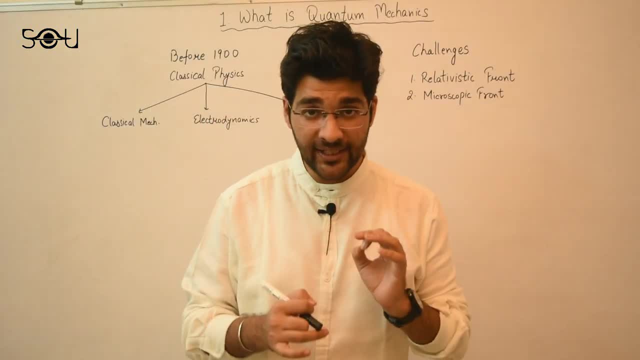 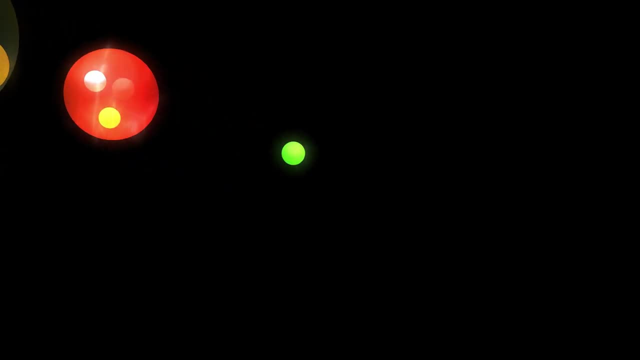 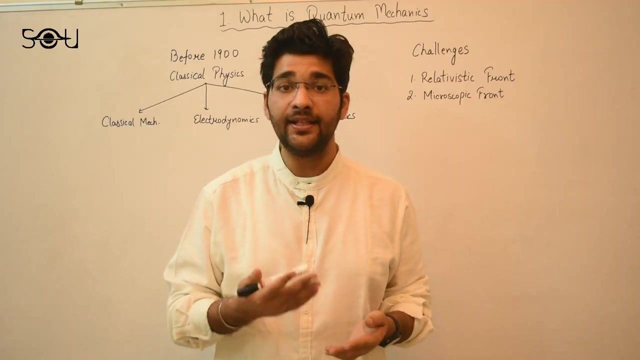 And second was on the microscopic front, When it was figured out that classical physics cannot even explain the dynamics at the microscopic level. It cannot explain the motion of the subatomic particles such as electrons. There were a series of experiments, For example the Young's double slit experiment, the blackbody spectrum, the photoelectric effect. 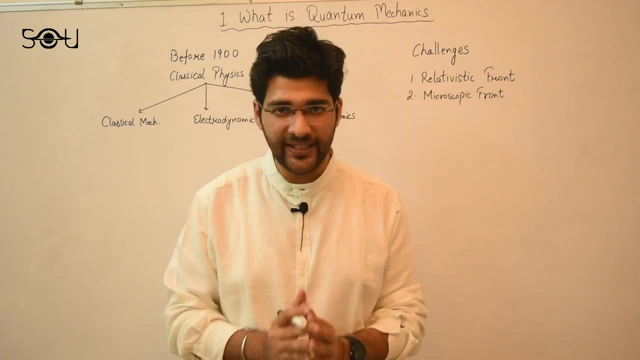 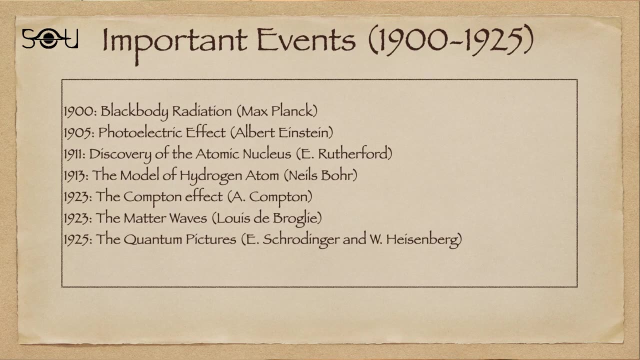 That could not be explained by classical physics. So it was very clear that we need new laws of physics to explain these phenomena. So I have prepared this small slide for you that shows some major events in the first quarter of the 20th century that led to the development of quantum mechanics. 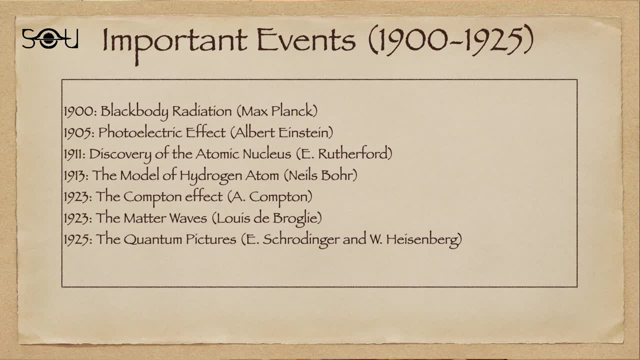 So we begin with 1900, when Max Planck explained the blackbody spectrum. This is where quantum mechanics formally began. Five years later, Albert Einstein used Planck's constant to explain the photoelectric effect, And then, in 1911, Rutherford discovered the nucleus. 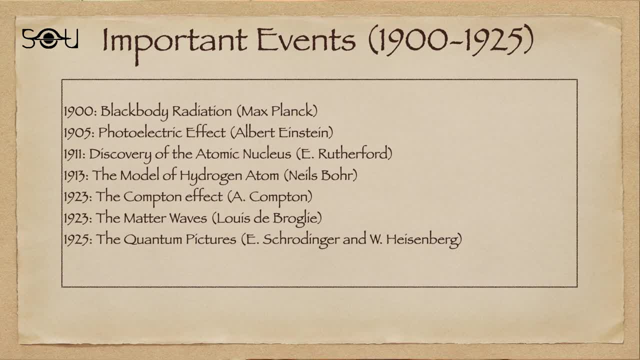 Two years later, in 1913, Bohr gave his atomic model, And then in 1923, we had the Compton effect by Arthur Compton. And finally, in 1925, Schrödinger and Heisenberg gave their own pictures of quantum mechanics. 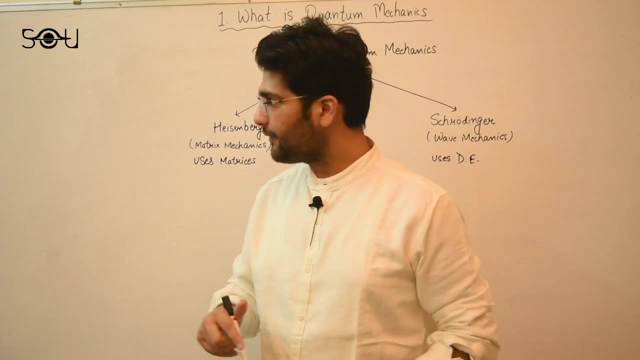 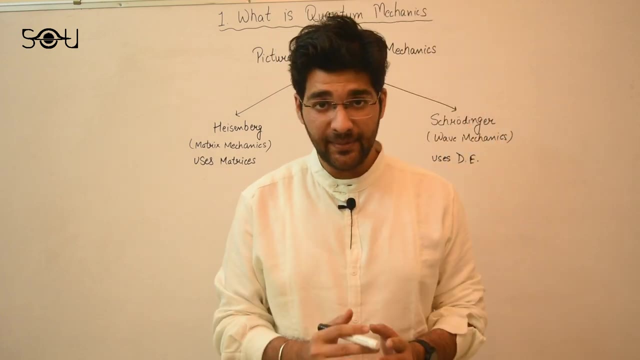 Historically, there are two pictures of quantum mechanics. The first is the Heisenberg picture, also known as the matrix mechanics. In the Heisenberg picture, dynamical quantities such as position, momentum, energy, etc. are described using matrices. 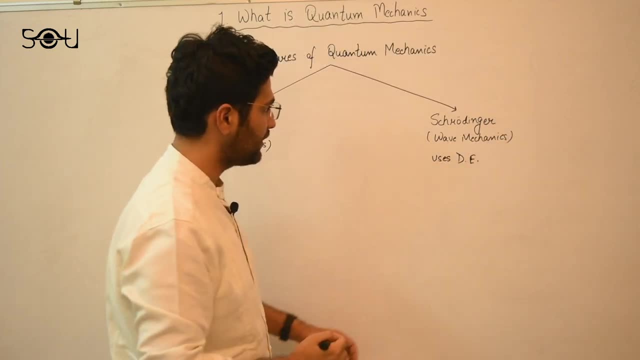 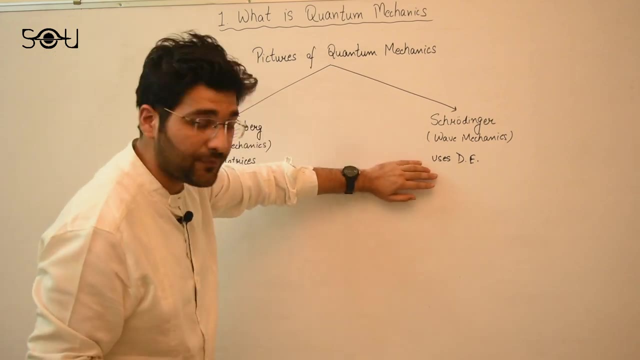 And then we have the Schrödinger picture given by Erwin Schrödinger. This is also known as the wave mechanics, And instead of matrices, Schrödinger's picture uses differential equations. This picture is more intuitive than Heisenberg's picture. 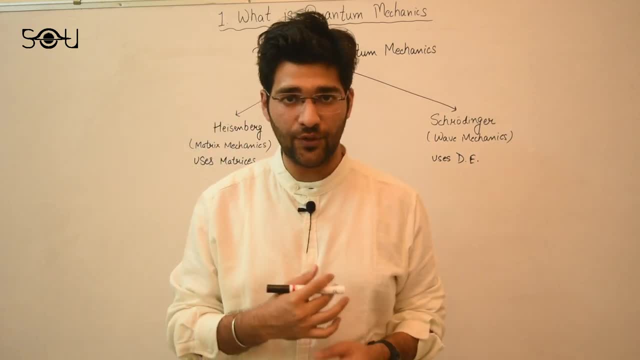 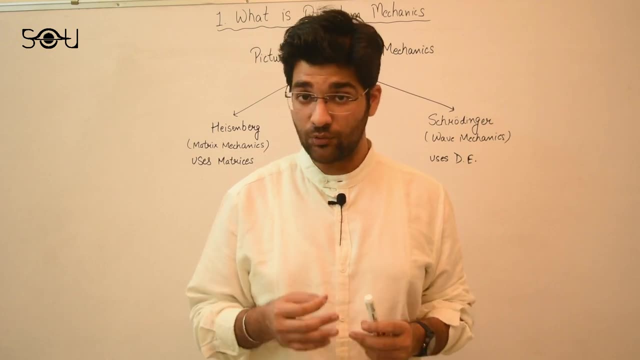 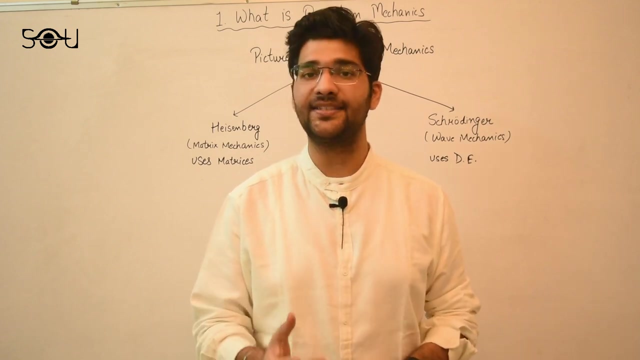 Later it was shown that both these interpretations of quantum mechanics, both these pictures of quantum mechanics essentially are the same. So you must have heard many people say that quantum mechanics is very difficult to understand. They don't understand it. And even Niels Bohr said: if quantum mechanics hasn't profoundly shocked you, you haven't understood it yet.